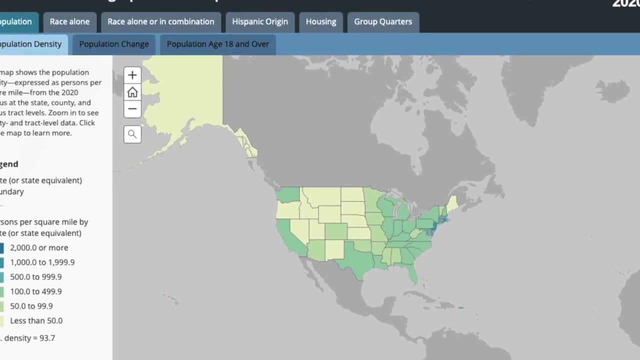 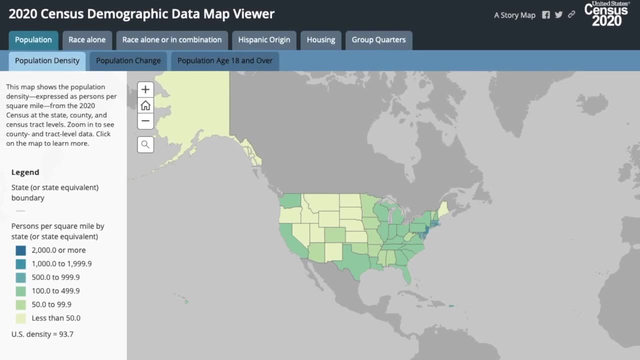 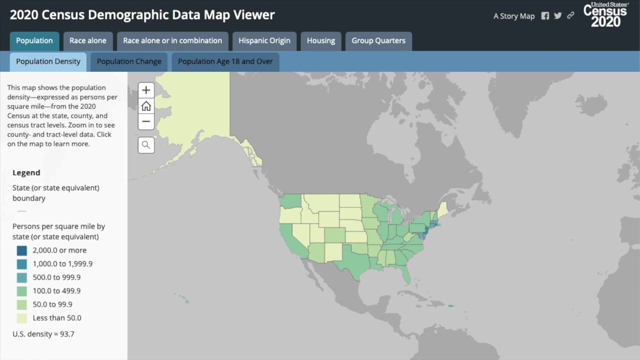 for tracks. This tool makes it easier for you to identify which tracks form your neighborhood. So let's start by visiting the 2020 Census Demographic Data Map Viewer. Click on the link on the right corner of this video or on the description of the video, Now that we are at the 2020 Census. 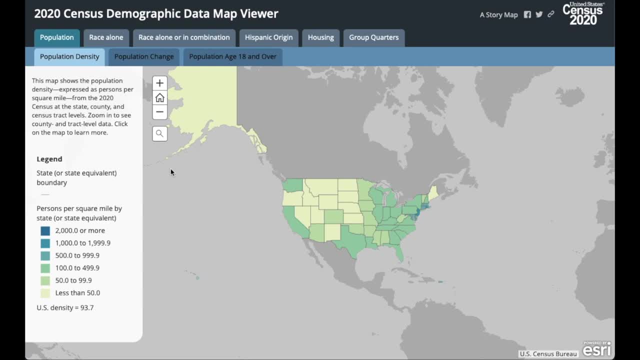 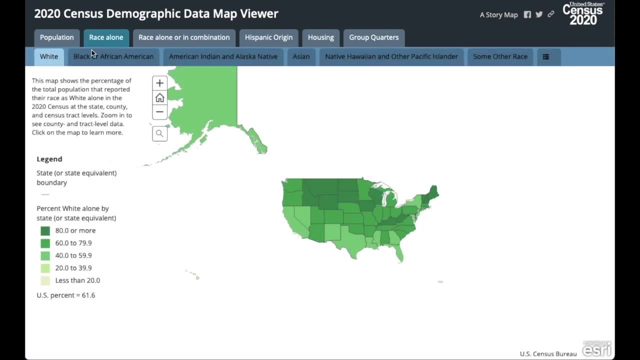 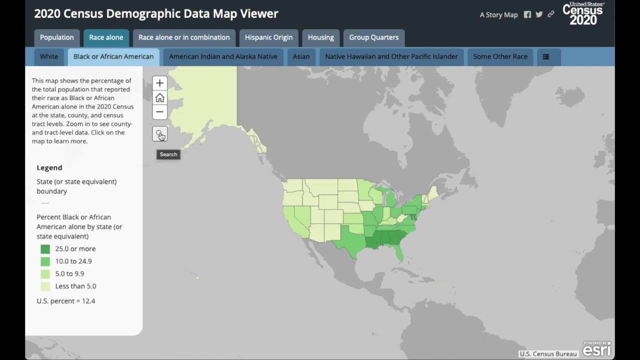 Demographic Data Map Viewer. let's first select a topic that you want to visualize data for your neighborhood. I will click on race alone. I will select black or African American to visualize. Now I'm going to conduct an address search. This is a great way to learn in which track 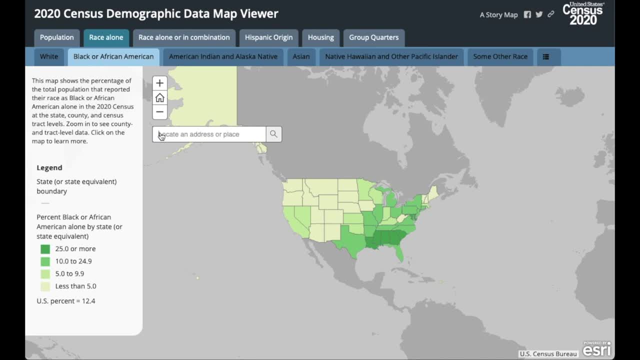 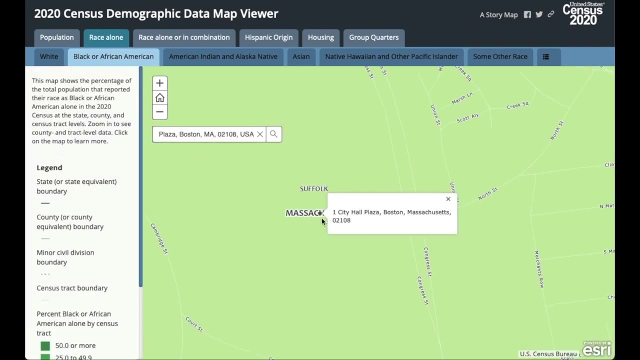 the address of your organization or service area is located. Let me take you to Boston, to a neighborhood that I'm very familiar with. I'll type the address: 1 City Hall Plaza in Boston. Now let's zoom out a little bit so we can see the boundaries of the track. 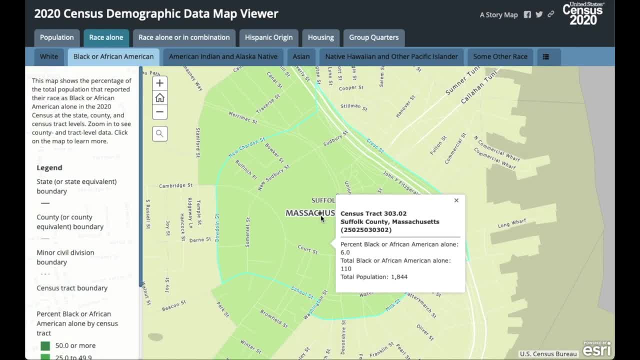 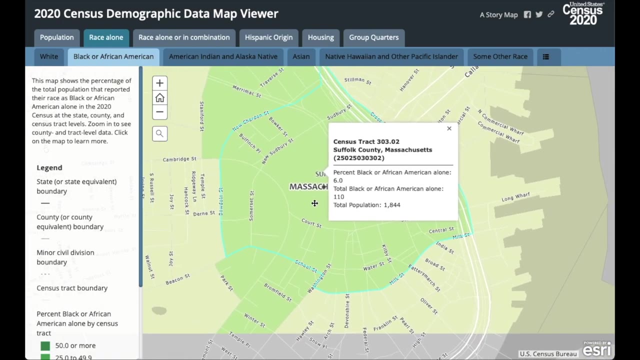 So if my neighborhood is the area of 1 City Hall Plaza, this address is located in Census Track 303.02.. If I click on the map, I can see the exact boundaries of the track and you can see the names of the streets to determine if this is the area of your neighborhood. 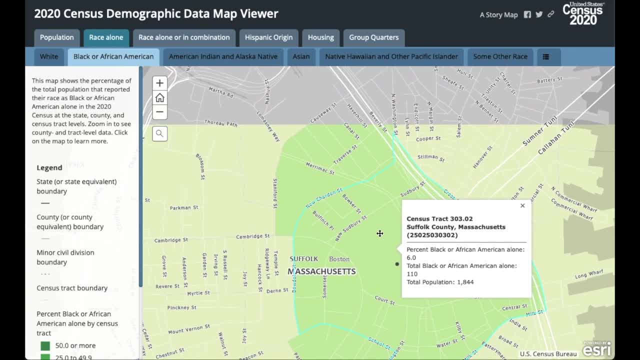 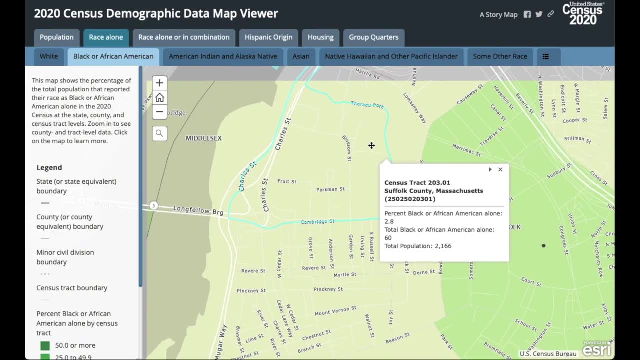 If your neighborhood is bigger than one track, you can keep selecting different tracks, one at a time, and don't forget to take a look at the streets that form the track. This will help you determine if the area is also part of your neighborhood. 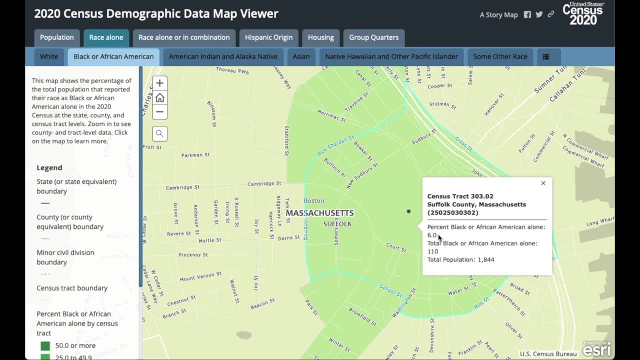 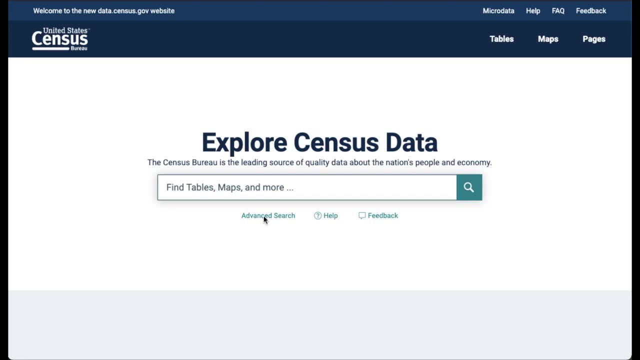 If you notice, once you click on a track, you get the data for that track. Next let's visit datacensusgov to access all the redistricting data tables for blocks and tracks. To go to datacensusgov, you can just type the address in your browser. 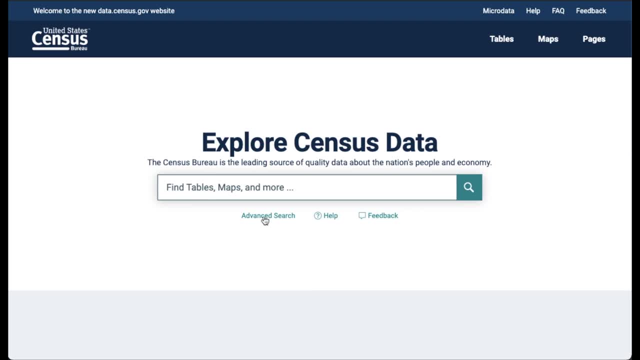 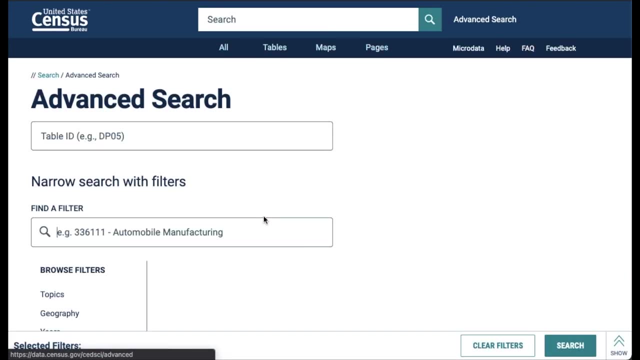 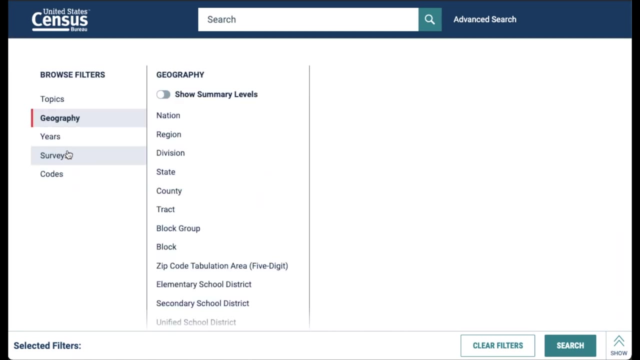 The recommended browser is Google Chrome. Now that we are at datacensusgov, let's start by going to Advanced Search. This is one of the many ways that you can access, block and track data. First, let's select our geography by clicking on Geography from the Browse filters. 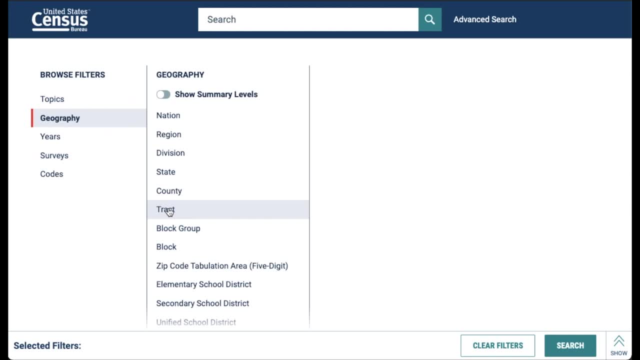 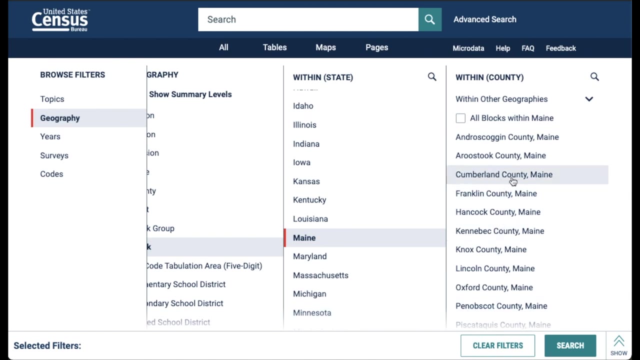 My geographic level will be block, but you could do the same thing here for a track. Select Block. Next, select the state of your block. I will select Maine. Next, the county of your block. I will select Cumberland County, Maine. 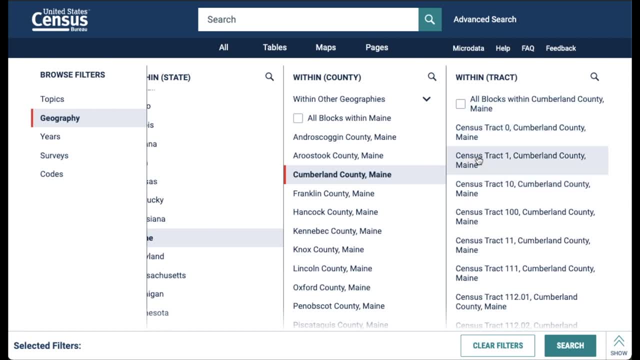 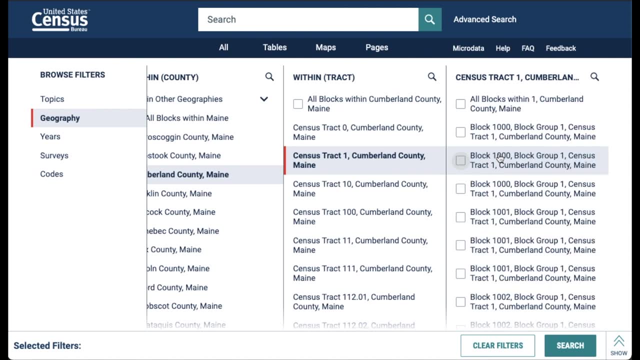 And I will select all blocks in Cumberland County in Maine. However, you could select blocks within a track, For instance, if you want to select Census Track 1, you see now the blocks within the census track And I can select them all one at a time. 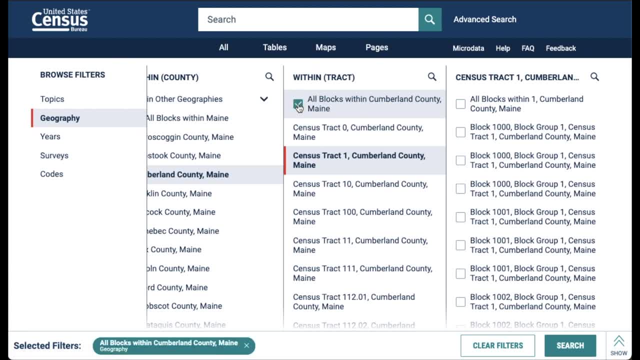 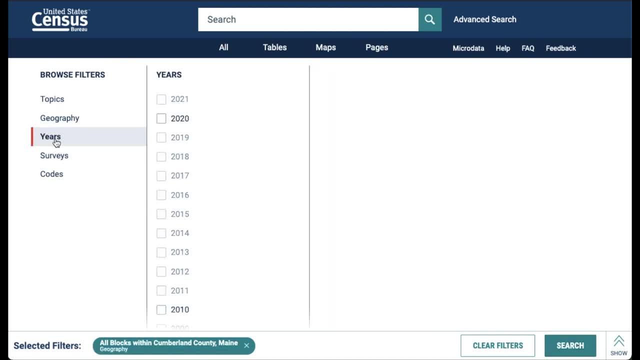 But I'm just going to go back to all blocks in Cumberland County in Maine. Next, to ensure that we only see data from the 2020 census, let's click on the year and select 2020.. You can also click on Surveys and select Decennial Census from the list. 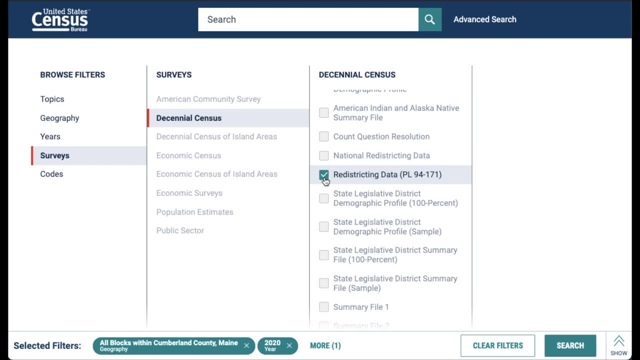 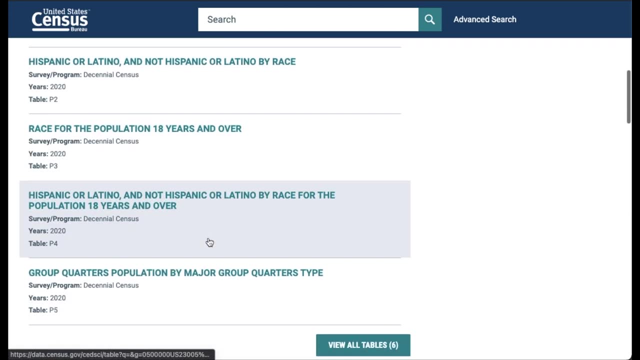 Next, select the tables from the Redistricting Data PL 94-171.. Now click Search and your results will be displayed. Next, select the tables from the Redistricting Data PL 94-171.. And your results will show tables from the 2020 census Redistricting Dataset. 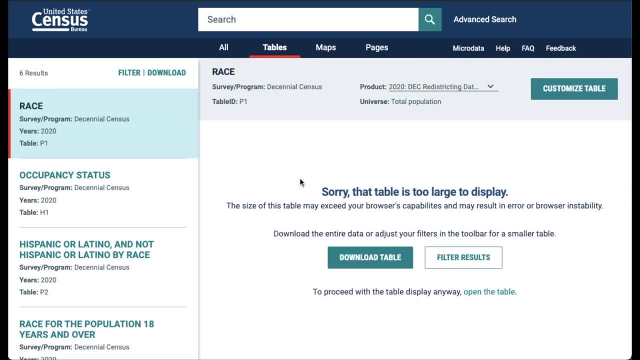 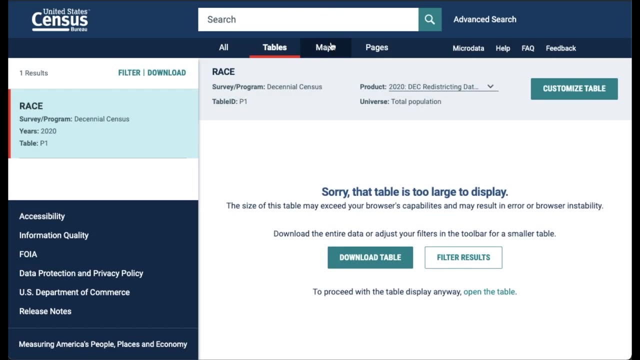 Let's open Table P1.. This system is not able to display the table results because of the large number of columns. However, to see the table, you can download it. Another great way to access this data is by visualizing it on a map. 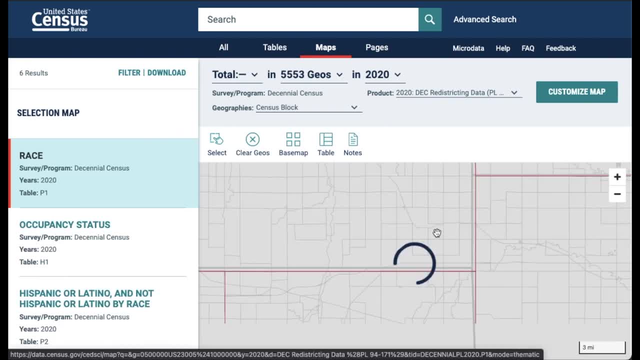 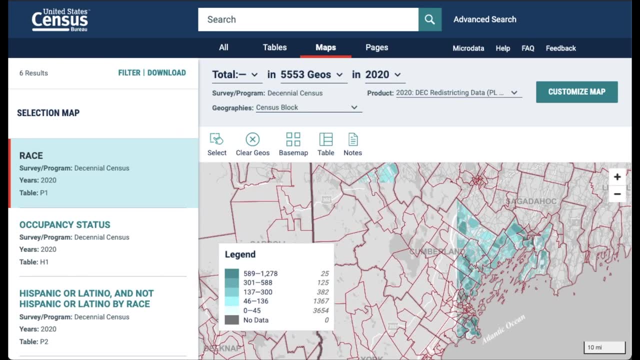 So let's click on Maps from the top menu. Once the map has loaded, I will select Table P1 and map the data from Table P1.. As you can see, the map for the county is now broken down by blocks and the data is displayed by blocks. 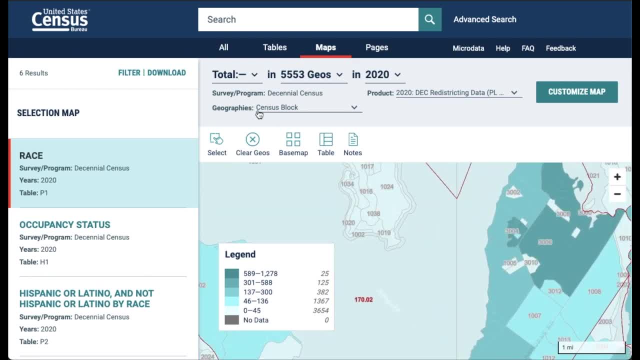 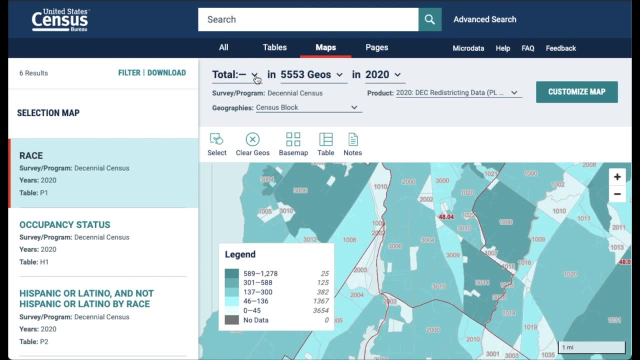 This can help you identify the blocks for your neighborhood and therefore you can see the data for your neighborhood. If you like to switch topics, you can click on the topic displaying from Table P1 on the map and switch from Totals to any of the topics available from the table.